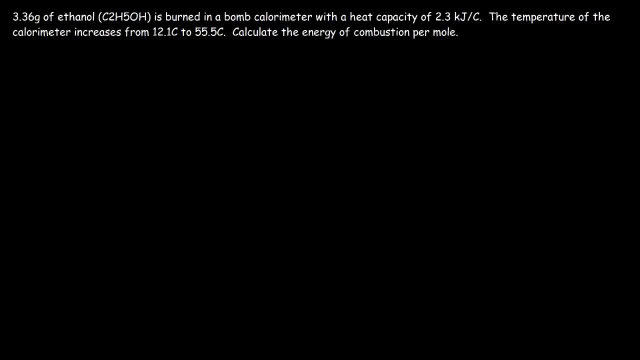 In this video we're going to talk about how to solve this bomb calorimeter problem. But before we go into it, I want to highlight the difference between the coffee cup calorimeter and the bomb calorimeter. So in the coffee cup calorimeter we're basically going to use a cup, ideally made up of styrofoam. 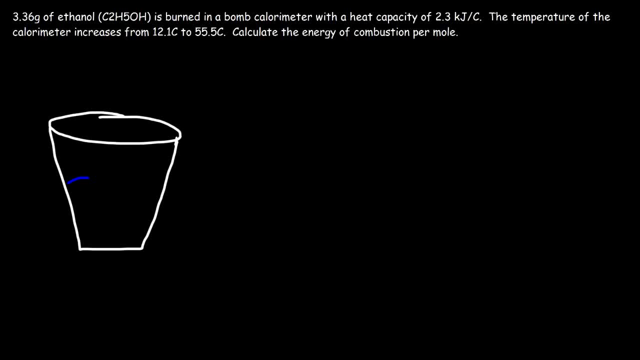 because styrofoam is a good thermal insulator. So we're gonna have some water in the cup and we need a thermometer to measure the temperature of the water sample And then we're gonna dissolve something into the solution. so maybe like calcium chloride And calcium chloride when dissolved in water releases. 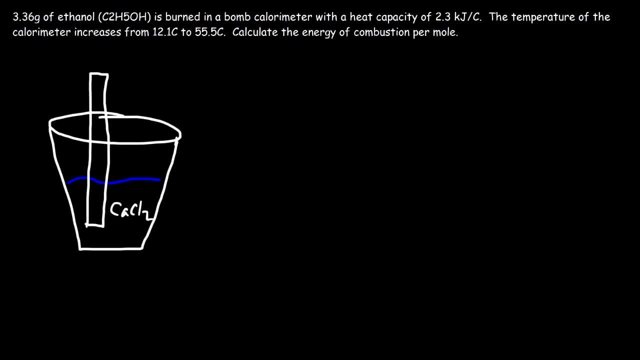 energy, And so the water molecules absorb that energy, and the temperature of the water is measured, And based on the change in temperature, you can calculate how much energy was absorbed by the solution, And so you can calculate the enthalpy change of calcium chloride. So this is the coffee cup calorimeter. 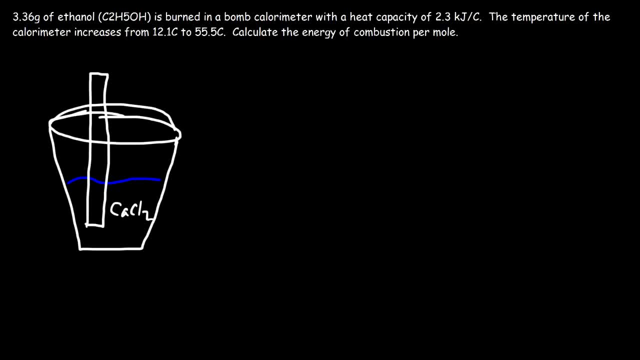 and it needs to be sealed Now. what you need to understand is that the coffee cup calorimeter measures the energy change at constant pressure. Because you have gas particles in the air, the pressure is going to be 1 atm at sea level Now. in a bomb calorimeter, the energy is calculated at constant volume. So why is 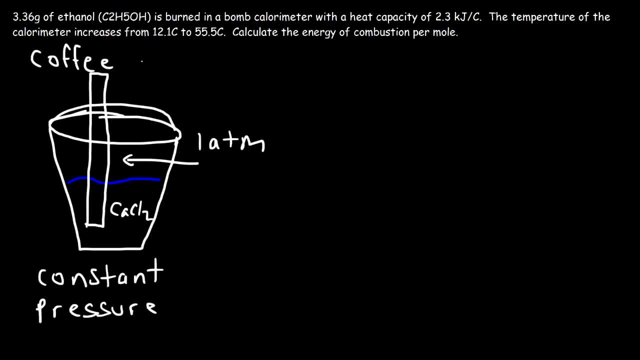 this important to know. This is important to know because enthalpy is the energy that is transferred only when measured at constant pressure. So if you wish to calculate the enthalpy of something, if we want to use the coffee cup calorimeter, You want to use the coffee cup calorimeter. 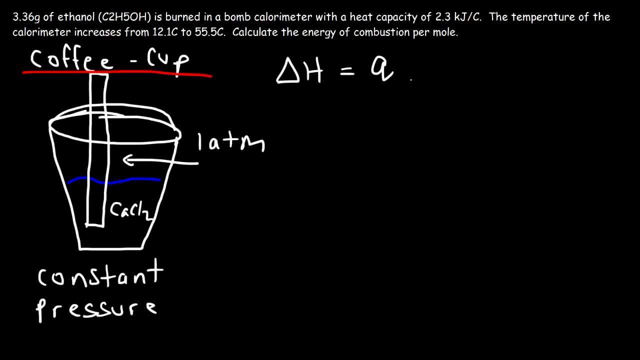 because the enthalpy change is equal to heat absorbed or released at constant pressure. Now in a bomb calorimeter the energy is measured at constant volume. so you don't want to use this to calculate enthalpy. That's why this question says: calculate the energy of combustion, not the enthalpy. 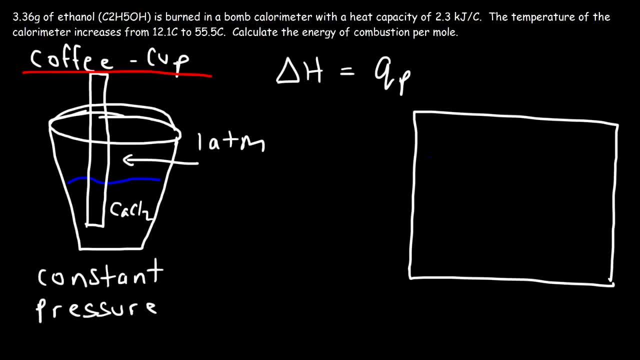 of combustion. Now, in a bomb calorimeter, you'll have water as well, so what you're going to use is some water, but you're gonna have a separate chamber, known as a combustion chamber- Let's put it on this side- and basically it's just a container that doesn't expand. It's a. 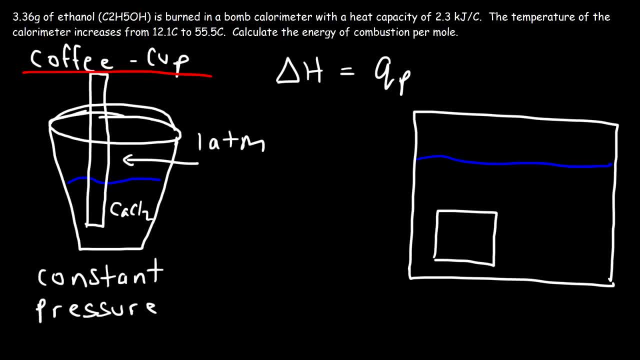 rigid container, and so the volume of that container is held constant. Now you're gonna have some ignition wires that extend from the combustion chamber to outside of the bomb calorimeter, and the purpose of the ignition wires is to basically ignite the sample. Once this sample is ignited, it's going to release. 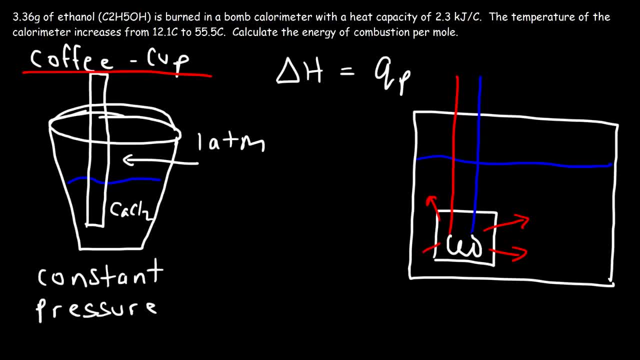 thermal energy into the surrounding environment, and so water is going to absorb that thermal energy, and so you need a thermometer to measure the temperature change of the water, And also you might have, like, some type of steering device to keep the fluid flowing, to transfer energy throughout the entire solution. So that's the 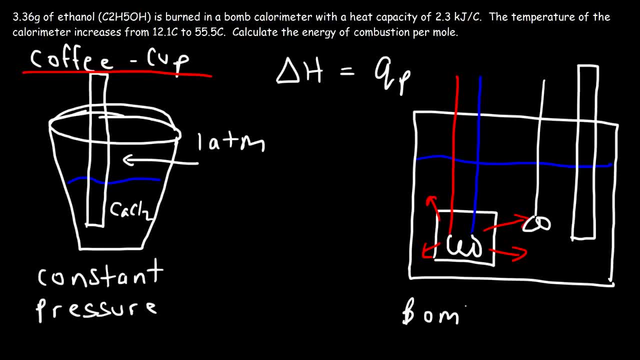 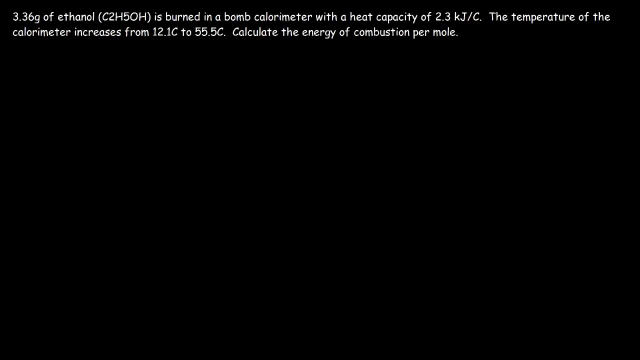 picture of the bomb calorimeter. It's similar to the coffee cup calorimeter, but you just have a combustion chamber, And just keep in mind that the energy changes are measured at constant volume. So that's important to know. So now let's focus on the problem at hand. 3.36 grams of ethanol is burned in a bomb. calorimeter with a heat capacity of 2.3 kilojoules per Celsius. The temperature of the calorimeter increases from 12.1 to 55.5 Celsius. Calculate the energy of combustion per mole. So how can we do this? The energy: 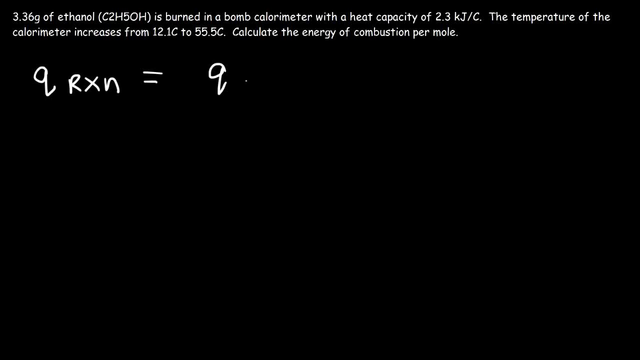 released by the reaction is equal to the energy absorbed by the water sample. Now how can we calculate this Q? Because we're not given the specific heat capacity of water. We know what it is, though: It's full Shuttle- 0.184 joules per gram per Celsius- but we don't know the mass of water in a sample. 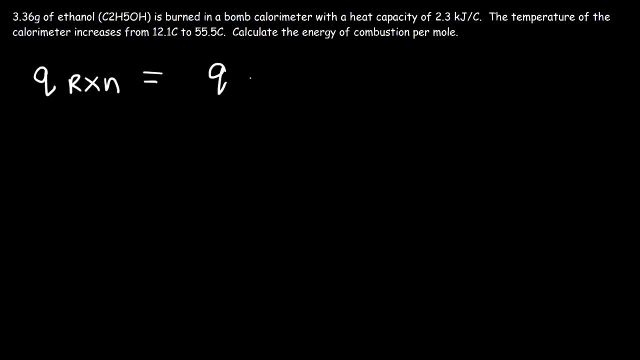 So we need to calculate the Q that's absorbed by the calorimeter as a whole, because we're given the heat capacity of the calorimeter. Now you need to be careful If you wish to calculate Q and you're given the specific heat capacity you need to use. 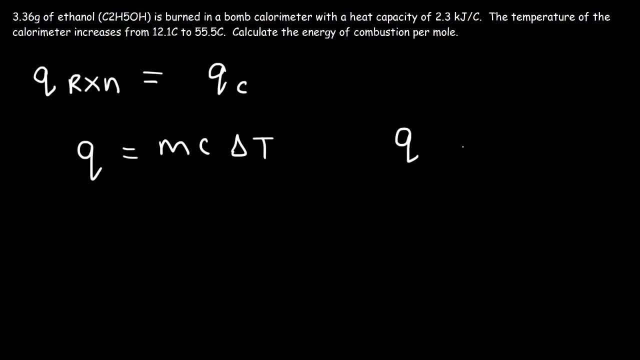 this equation mc delta T. But if you're given the heat capacity, it's simply c delta T And the units basically tell you that. Notice that for the heat capacity the units are kilojoules per Celsius. So if we multiply kilojoules per Celsius by the temperature change in Celsius, it's going. 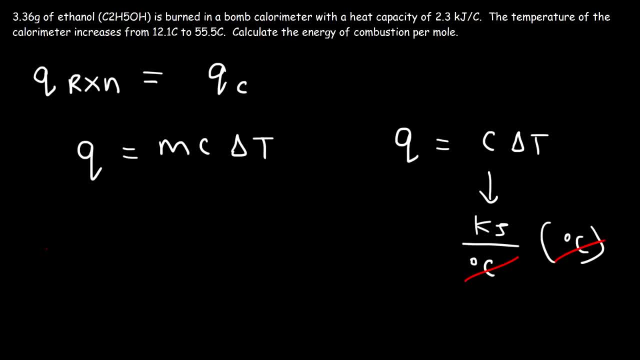 to give us the energy in kilojoules, which we're going to divide it by moles later. But when you're dealing with specific heat capacity, c is going to have the units joules per gram per Celsius, And so you need to multiply c by m so that the unit grams will cancel. 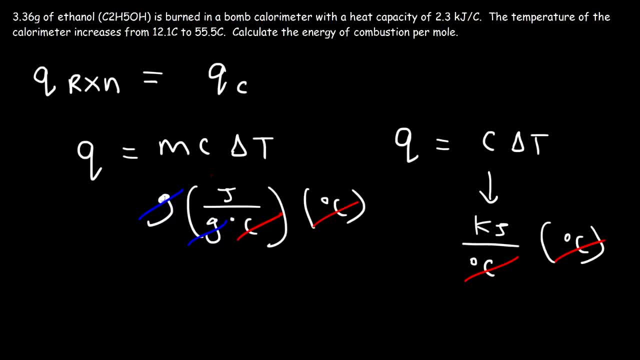 And once you multiply by delta, T Celsius will cancel giving you joules, Or this could be kilojoules too as well. So now let's go ahead and calculate the heat energy that's absorbed by the calorimeter. So that's going to be the heat capacity. 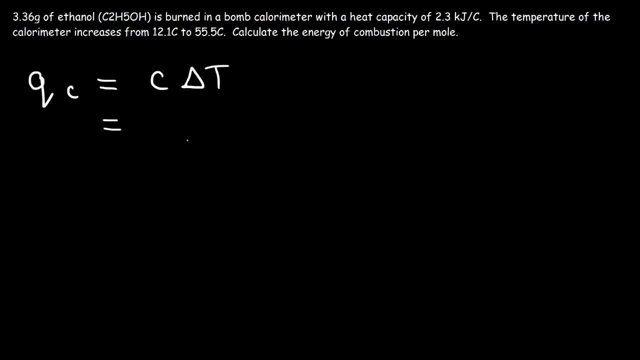 Multiplied by the change in temperature, The heat capacity is 2.3 kilojoules per Celsius And the change in temperature it's final minus initial, So that's going to be 55.5 minus 12.1.. 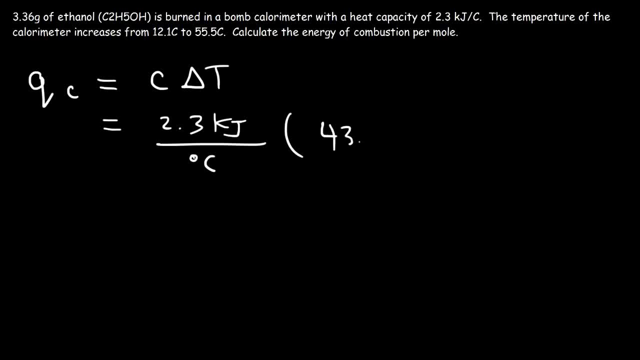 So that's a change in temperature of 43.4 degrees Celsius. So if we multiply 2.3 by 4.1. That's going to be 2.4.. And if we multiply 2.4 by 4.1., 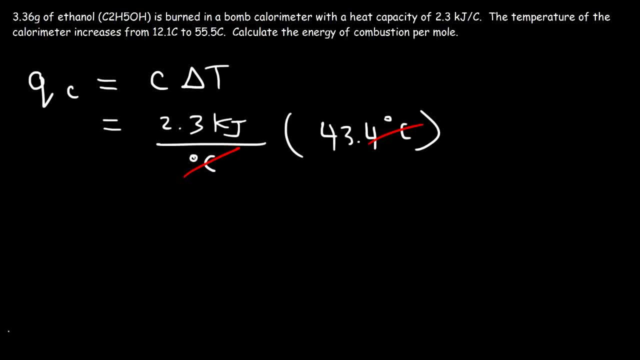 That's going to be 2.5 minus 5.1.. And that's going to be 2.4.. 43.4 that gives us 99.82 kilojoules and because the temperature of the calorimeter increased, we could say that the process is endothermic for the. 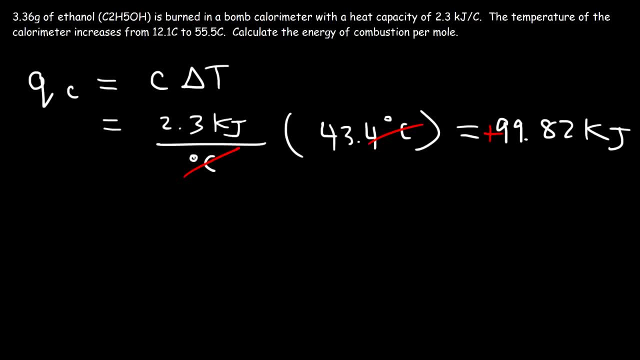 calorimeter. heat was absorbed by the calorimeter, which means that heat had to be released by the reaction. so Q of the reaction is equal to negative Q of the calorimeter. The calorimeter is the surroundings, the reaction is the system. so if the surroundings is undergoing an 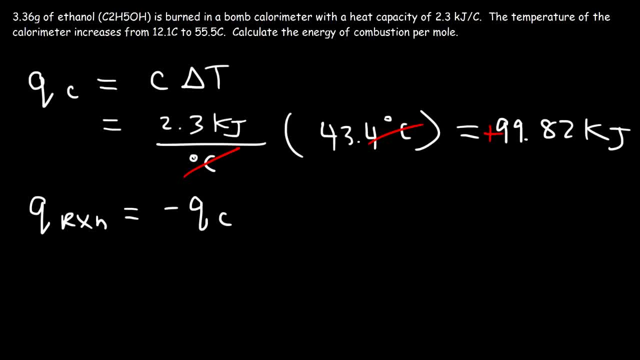 endothermic process. the system has to be undergoing an exothermic process. so Q of the reaction is negative: 99.82 kilojoules. Now we need the energy of combustion per mole, so we have the grams of ethanol. we need to convert that to. 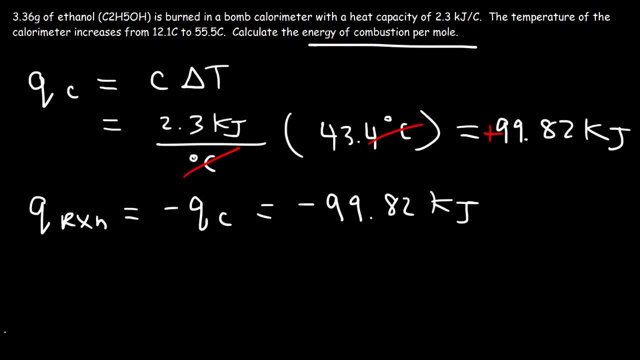 moles. but let's calculate the molar mass first. So in ethanol we have two carbon atoms, a total of six hydrogen atoms- 5 plus 1 is 6, and then just a single oxygen atom. So the atomic mass of carbon is 12.01, and the atomic mass of hydrogen is 1.008, and 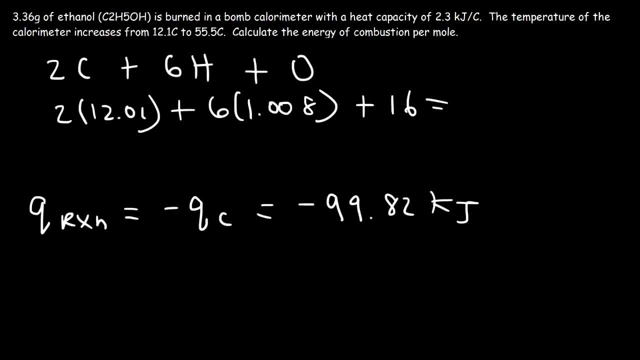 oxygen is 16.. So type that in exactly the way you see it in your calculator. So you should get a molar mass of 46.068 grams per mole. So let's start with 3.368 grams per mole, 46 grams of ethanol, and let's convert it to moles. 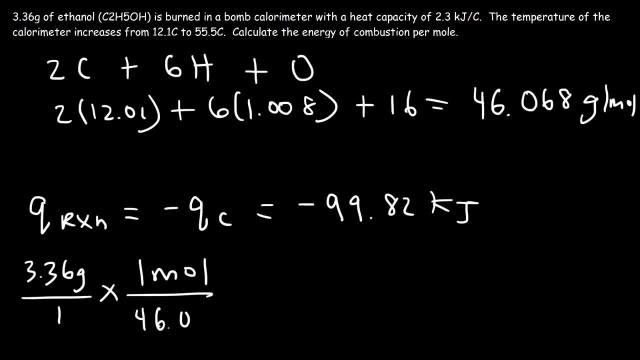 So to calculate the number of moles you just simply have to take the mass and divide it by the molar mass. So it's 3.36 divided by 46.068.. And so this is going to be 0.0729 moles. 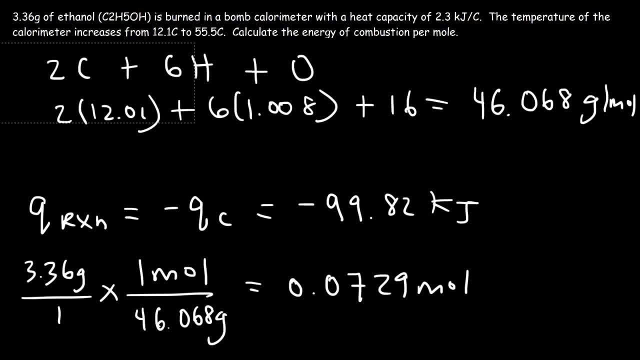 So now, to calculate the energy of combustion per mole, we need to take the energy in kilojoules and divide it by the number of moles. So it's going to be negative 99.82 kilojoules divided by 0.0729 moles. 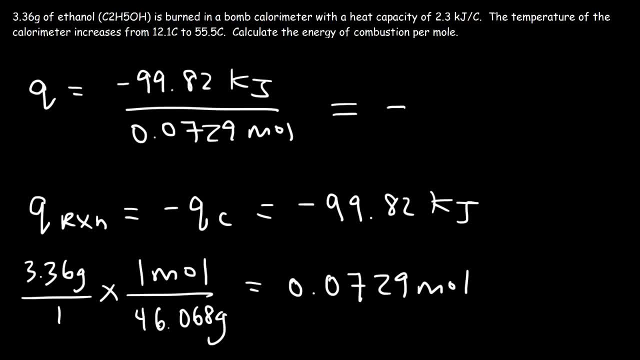 So it's going to be about. if you round it to 3 sig figs, it's negative 1370 kilojoules per mole: 0.0729.. So that's the energy of combustion per mole for the substance ethanol.